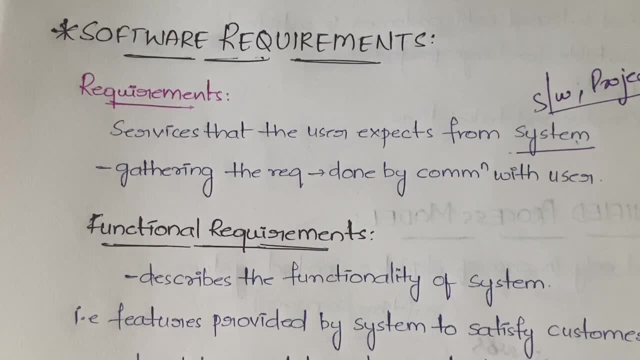 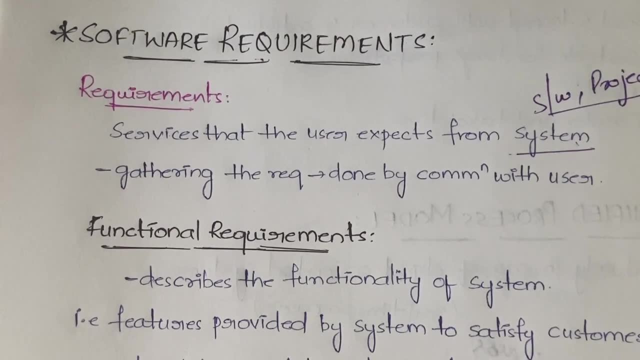 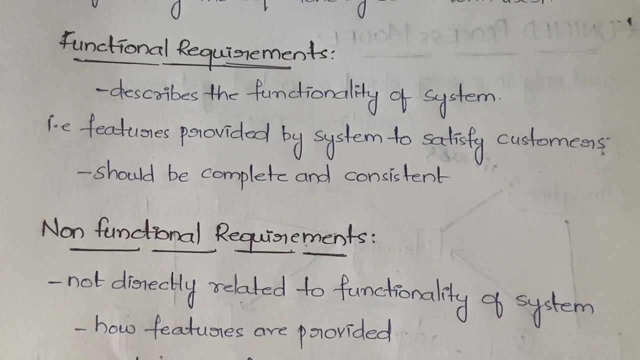 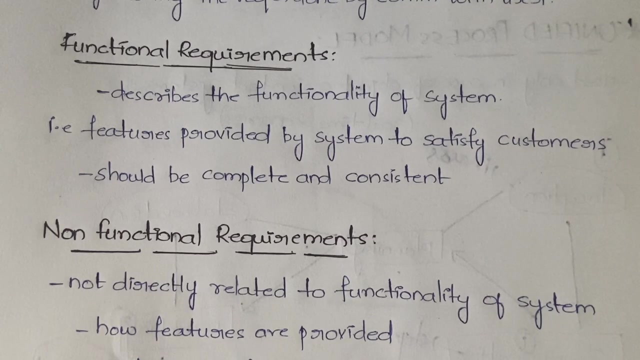 Functional and non functional. This is based on the functionality. We again have user requirements, system requirements and all, But this is based on the functionality of the system. We have two types. Okay, so let us see those two things. The next categories I'll explain in the next video. First is a functional requirements. Functional requirements- simple. they will describe the functionality of the system. functionality of the system in the sense how the system is work. Sorry, sorry, sorry, not how the system is working. What are the functional requirements? 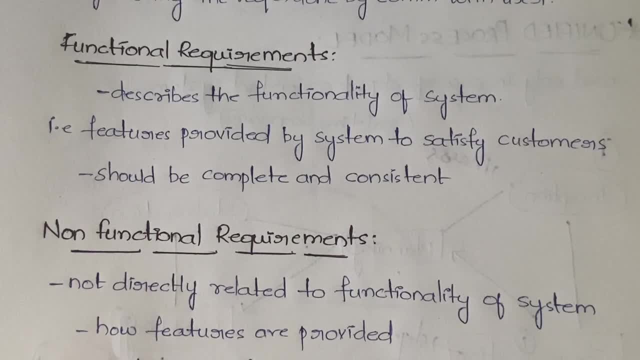 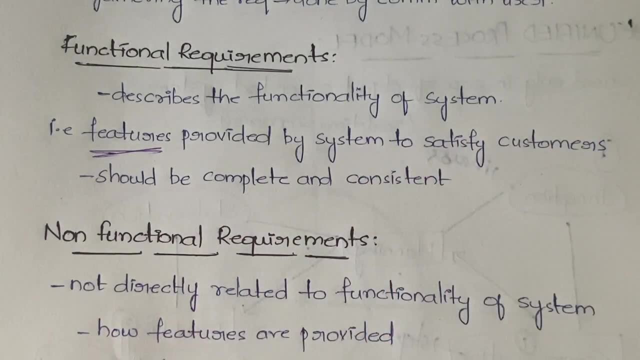 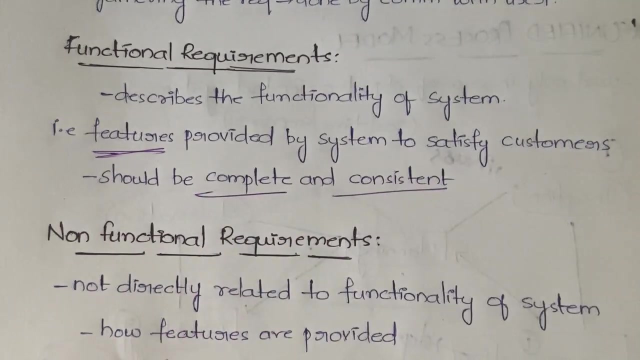 That are provided by the system, that will be given by the functional requirements, That is, the. what are the features that are provided by the system in order to satisfy the customers. and these functional requirements should always be complete and complete. by complete, That is all services which the user is expecting. All those should be satisfied. and consistent means like the requirements should not have any contradictions. Okay, so complete means. 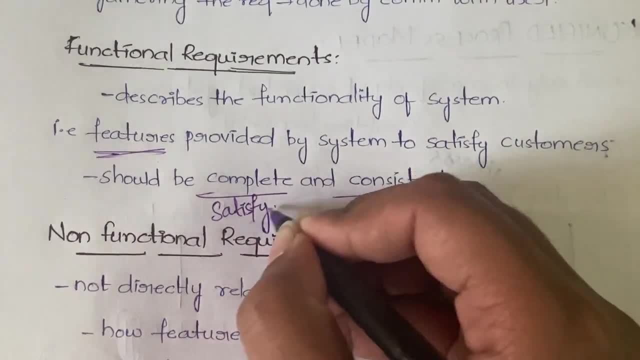 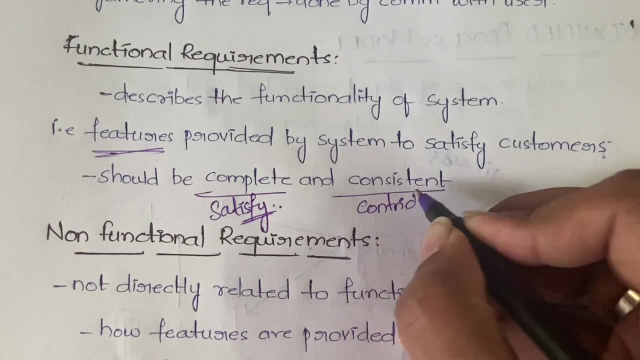 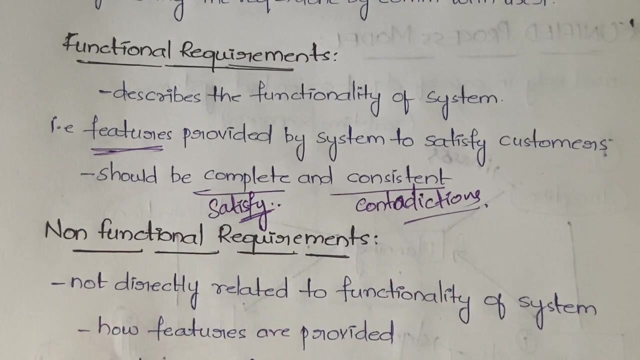 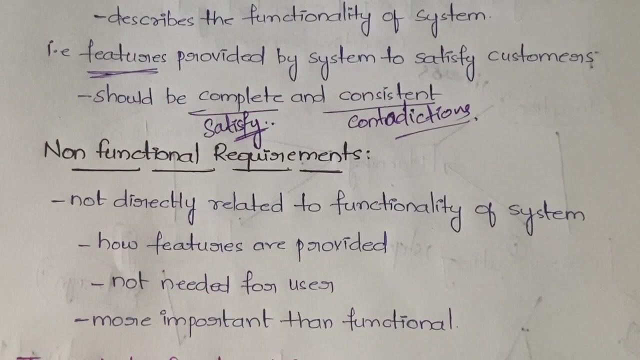 the. all the requirements that the user is requesting should be satisfied and consistent, in the sense the software should not have any Sorry contradictions. right Contradictions? Okay done, Sorry, requirements should not have any contradictions. Next. So this is about the functional requirements. Next, non functional requirements. in functional, you don't have any further subcategories. Okay, in non functional requirements. 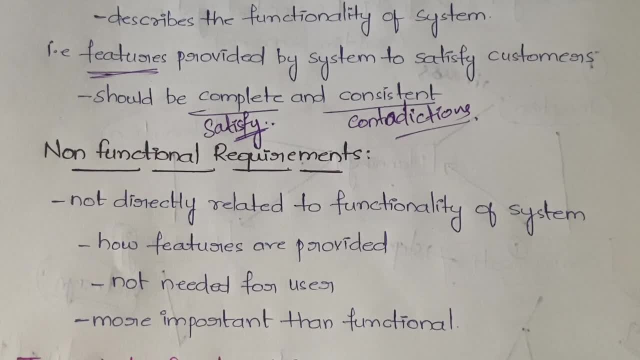 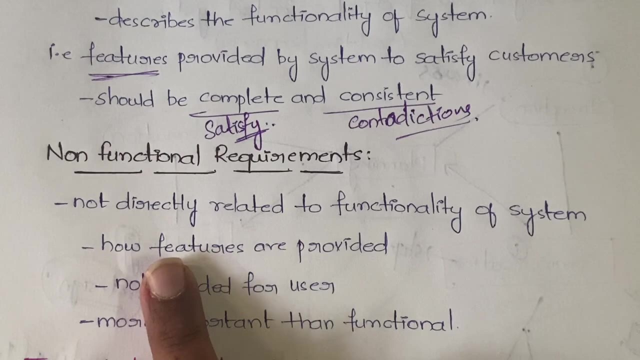 They are not directly related to the functionality of the system. Okay, that means They, the non functional requirements, will not show you the features which are given by the system, But what they will show. they will show how those features are provided here. 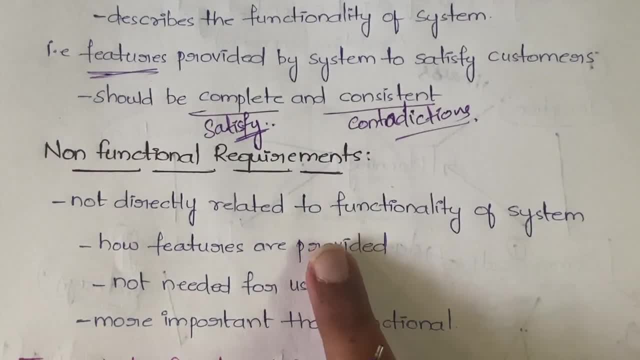 Only the list of features is provided, but here it will show the implementation of those features as well. That is how you are implementing those features. Got it, Got it. Got it about the non-functional requirements, and these non-functional requirements are not needed to the. 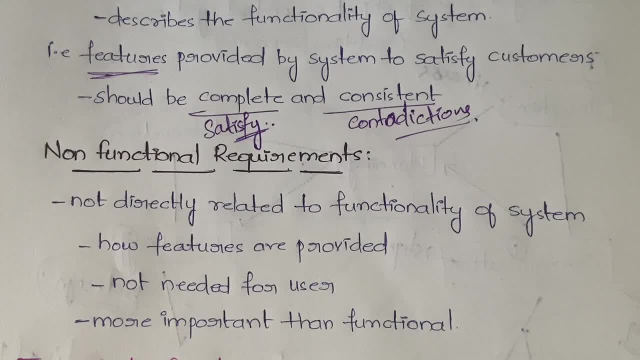 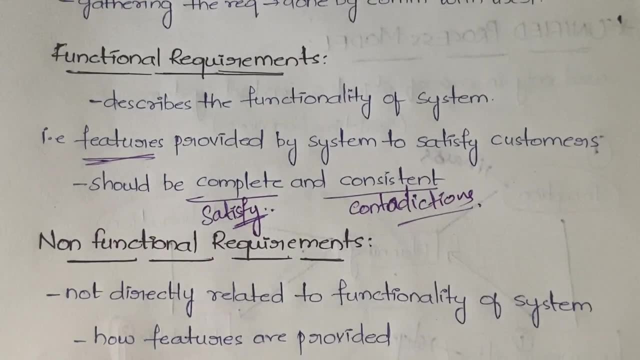 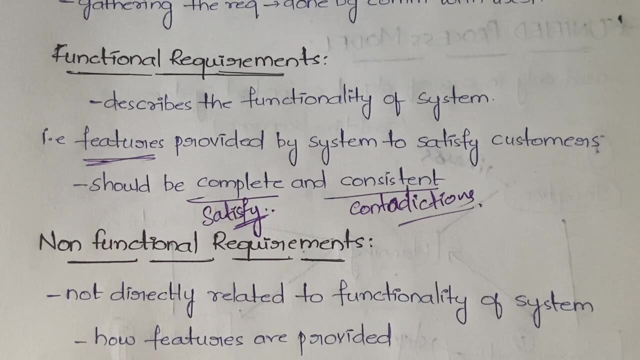 user and they are very important when compared to the functional requirements. done got it. so main thing is: what is the difference between functional and non-functional? functional will give you the features which are provided by the system, whereas non-functional will explain you how those features are provided that is not needed for the customer. okay, they are abstracted and we 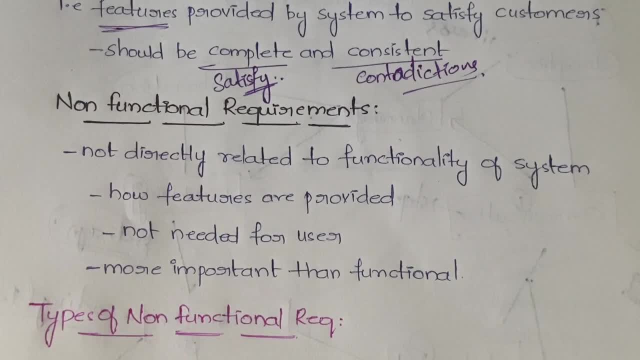 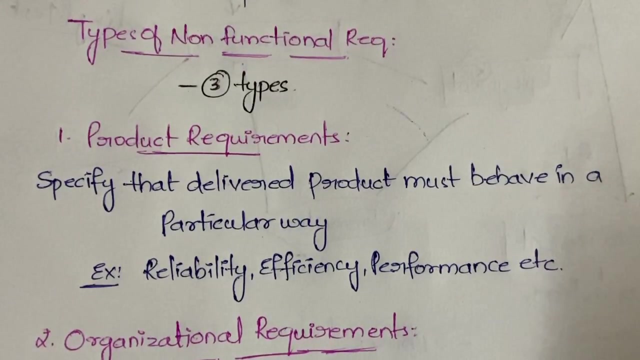 have different types of non-functional requirements. under functional we don't have any subcategories, but in non-functional we have. so we have three subcategories. let us now understand what are those three subcategories. in non-functional requirements we have three types: product requirement or requirements, organizational requirements and external requirements. 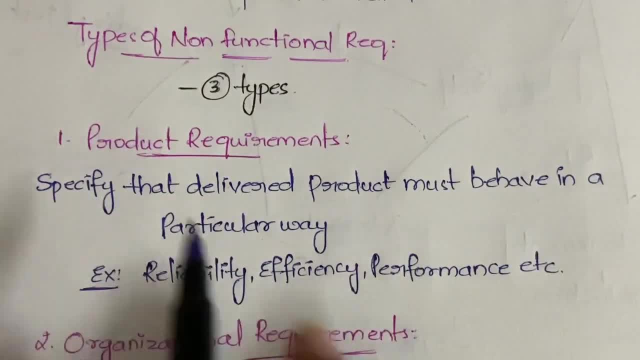 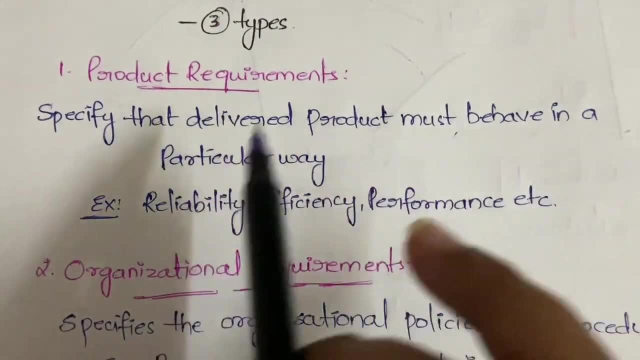 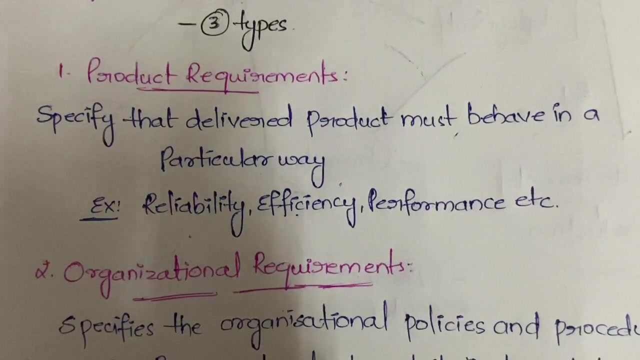 so let us see what each of them is. first, product requirements. what product requirements will do is they will specify that the delivery product must behave in a particular way, that is, it has to have reliability, it has to have so and so efficiency, it has to give so and so percent, uh, performance. like that it will give you the product. 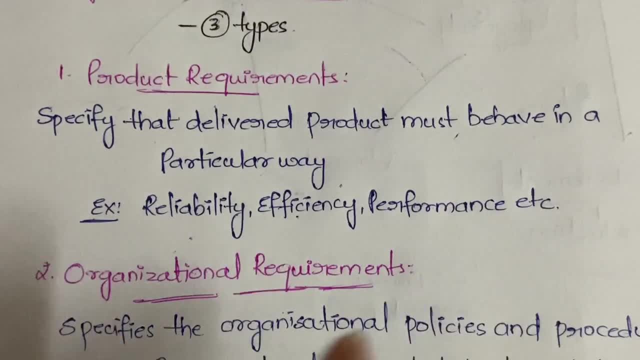 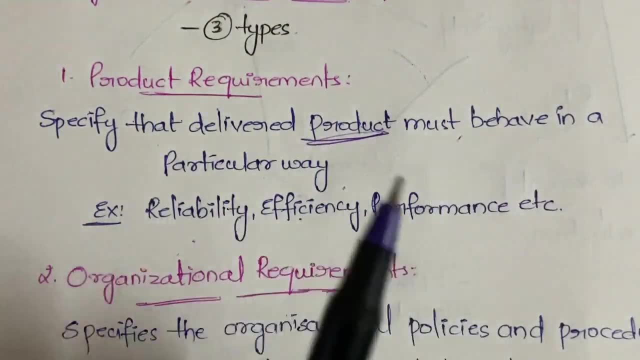 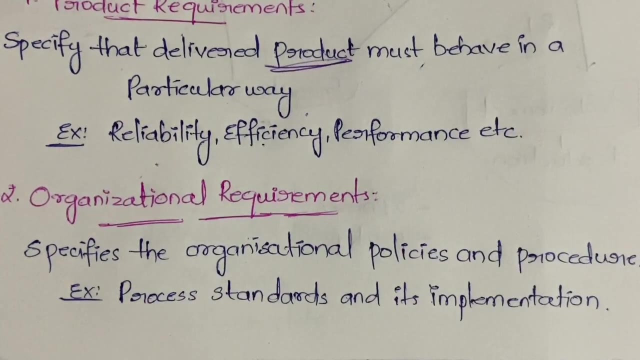 requirements will give you the- uh, you know- measures we can say. it will specify the delivered product, that is, the delivered software must have, uh, so and so qualities. okay, that is about the product requirements. the next is the organizational requirements. so, uh, in organizational requirements, it is very simple again, it specifies that is the requirements, uh, that are that will specify the 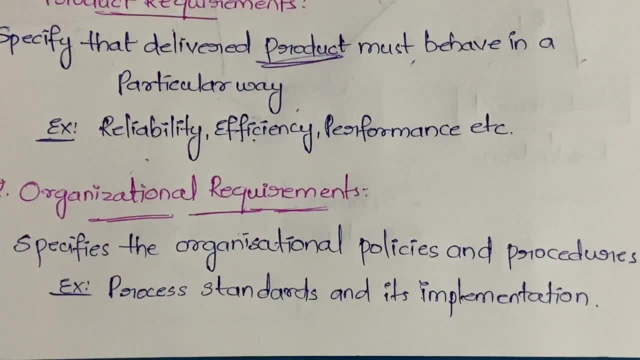 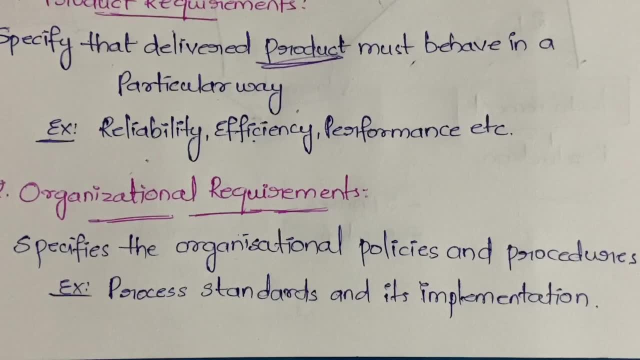 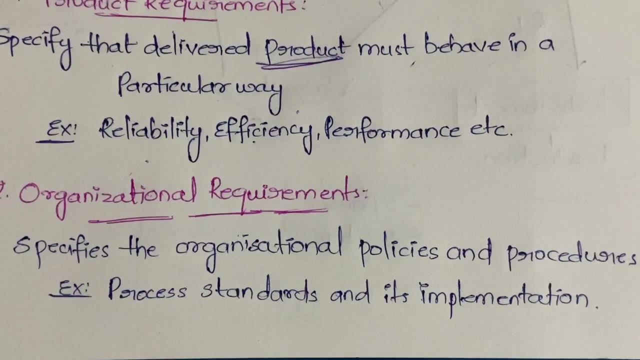 organizational policies and procedures. that is, if you are working in an organization, that organization will have some rules, right suppose, in a college we have some rules, right like um, no ragging, you should not carry cell phones, and also you have some rules. so the organization also will have some rules. so the requirements which will specify the organization's policies, procedures, 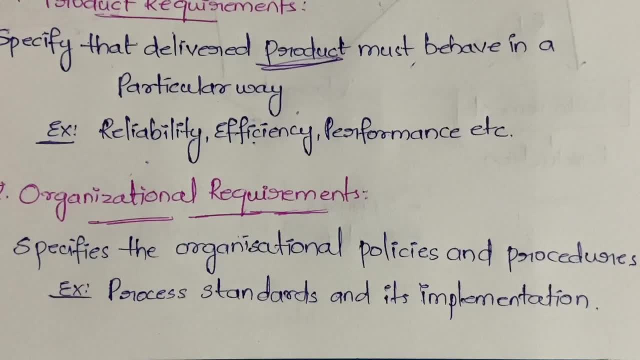 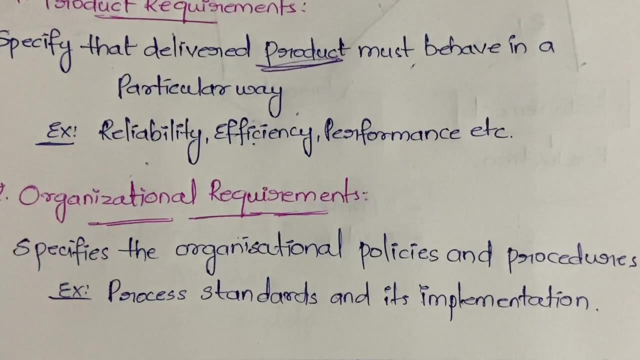 under the organizational requirements. got it, for example, process standards and its implementation. that is, you are, you know, defining a process or a project or a product or software, whatever it is. what are the standards that the product have to maintain and how do you implement those standards? got that is about the organizational requirements. right next, after organizational requirements, the